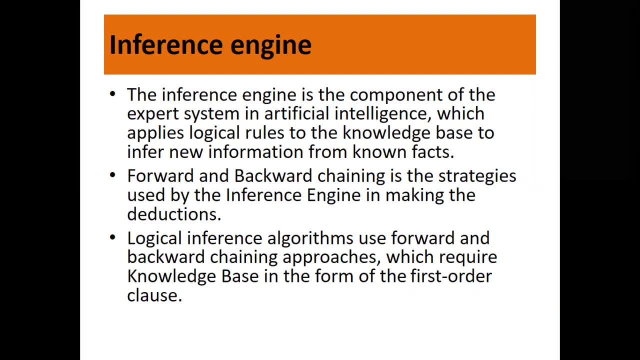 rules to the knowledge base, to infer new information from the known facts. So here the set of rules are stored and the facts are given where matched with the rules and accordingly the output is given. So forward and backward chaining is the strategies used by the inference engine in 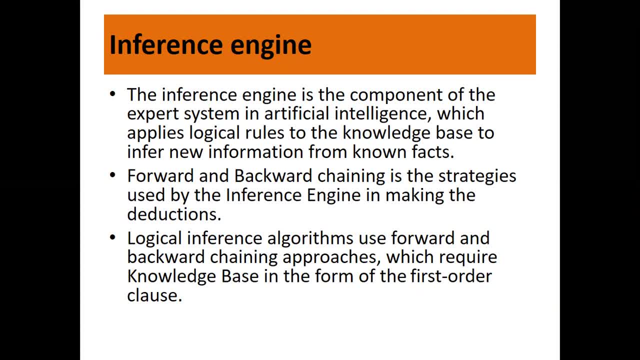 making the deductions. Logical inference algorithms use forward and backward chaining approaches, which requires knowledge base in the form of first order logic. We already know we have worked a lot with first order logic and we know the knowledge base contains the facts and uses the knowledge base in the form of first order logic. So we are going to look at the 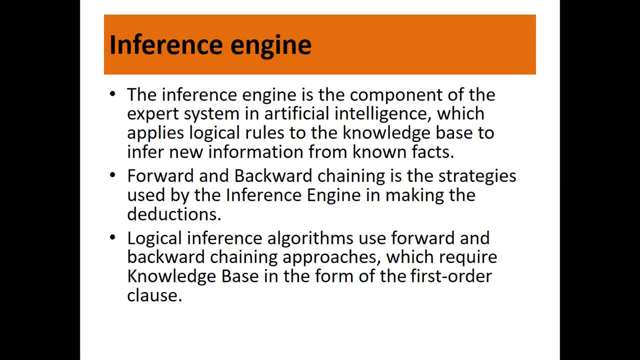 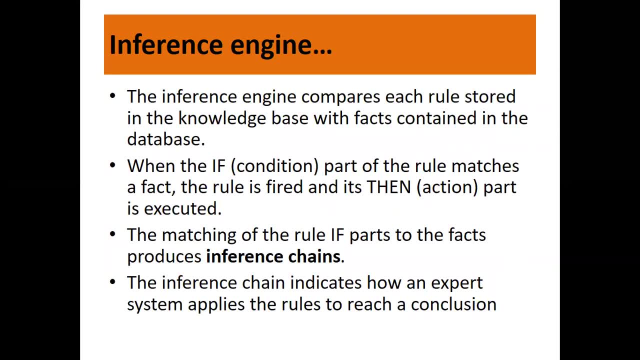 those facts, you apply inference techniques to generate a new fact. Now the inference engine compares each rule stored in the knowledge base with the facts contained in the database. Rules are stored in the knowledge base and the facts are. facts are nothing but the statements, single statements. right, They are compared with the rules When? 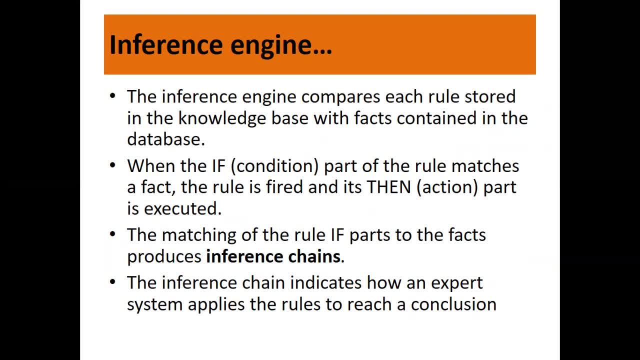 the if condition, that is, if part of the rule matches the fact, the rule is fired and it's then action part, that is, it's then part is executed right. So if else rule is taken from the knowledge base, the fact what is given is taken If the fact. 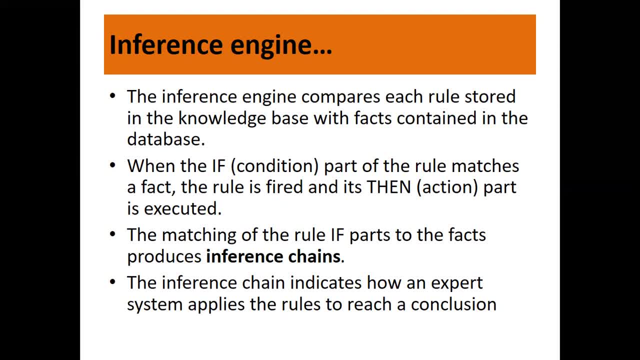 is part of the if condition what you write in front of the if. if it is matching, then the then part of that if condition is executed. The matching of the rule if parts to the facts produces inference change. So we'll look at inference chain also in the next slide. The 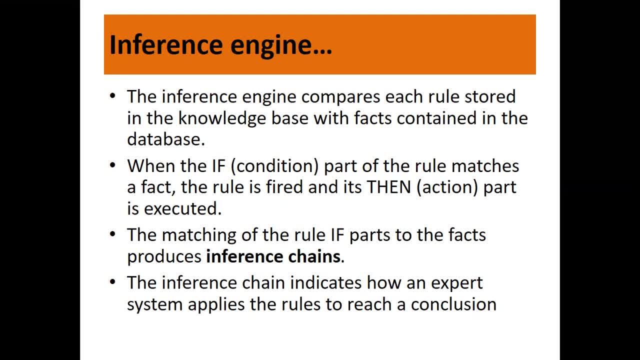 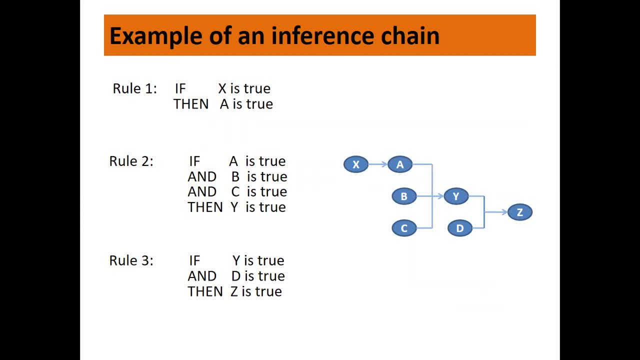 inference chain is the rule that is given to the facts. The rule that is given to the facts produces inference. The inference chain indicates how an expert system applies the rules to reach a conclusion. So let us look at the example of inference chain Here. suppose these are. 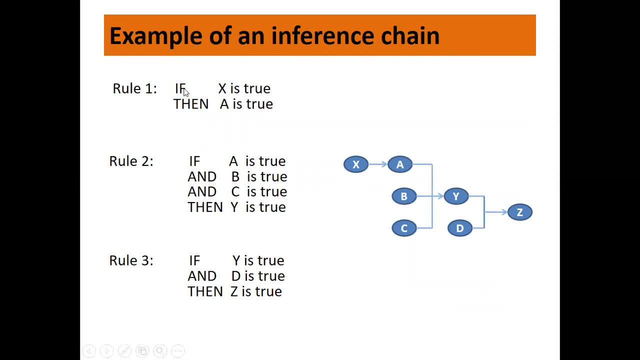 the three rules which are already stored in the knowledge base And as I set the rules, if, if and then or if, then These are the rules. There are three rules. What rules first says: if X is true, then A is true. If X is true, then A is true. that X implies A. if X is true, then A is true. 3. pleasure familiar with references. ordering doesn't matter whether it's a true or a false. in our scenario, three rules. What rules first says: if X is true, then A is true. that X implies A. if X is true, then A is true. 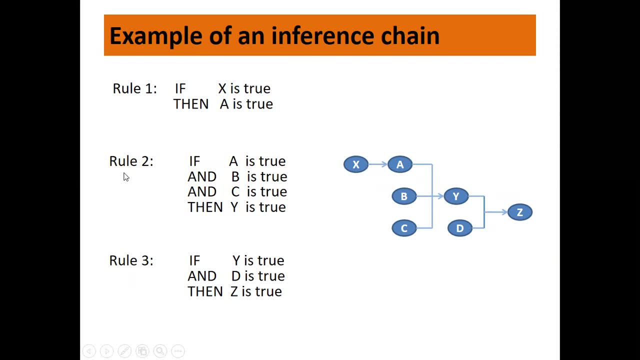 A. If X is true, then A is true. What the second rule says: if A is true, B is true, C is true, then Y is true, right? So if A, B and C, all these three are true, then Y is true, fine. 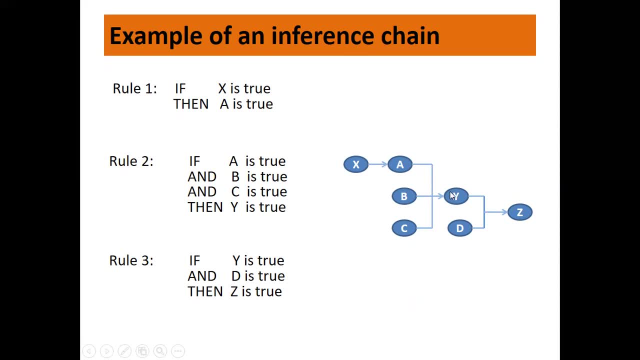 Just look at the chain from this you are moving ahead. this right What the rule 3 says: if Y is true and D is true. if Y is true and D is true, then Z is true, right? The simple example of. 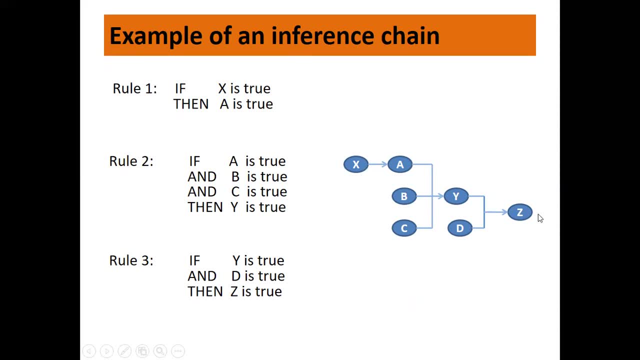 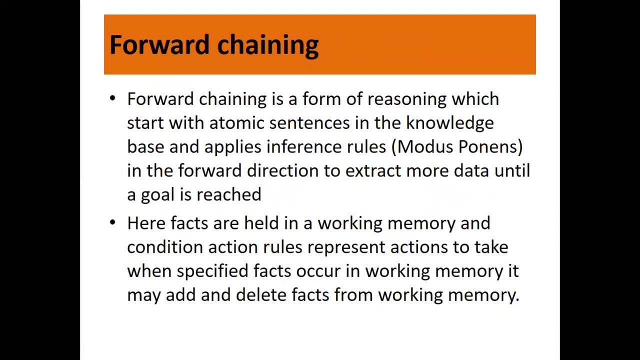 inference chain. Let us look at forward chaining in detail. Forward chaining is a form of reasoning which starts with atomic sentences in the knowledge base and applies inference rules. We already studied inference rules in the previous lecture videos. If you have not gone through it. 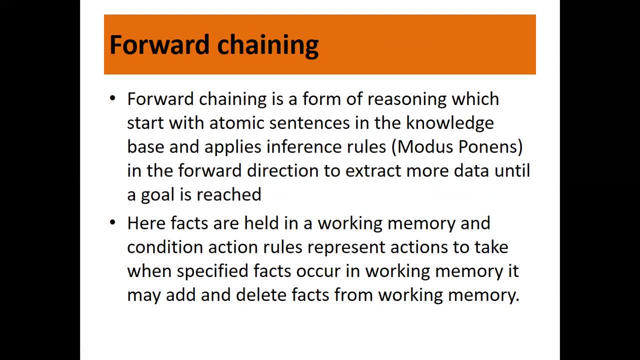 please go through it, And especially here. modus ponens will be used in the forward direction to extract more data until the goal is reached. Here. facts are held in a working memory, and condition action rules represent actions to take when specified fact occurs in the working memory. it may add and delete facts from the 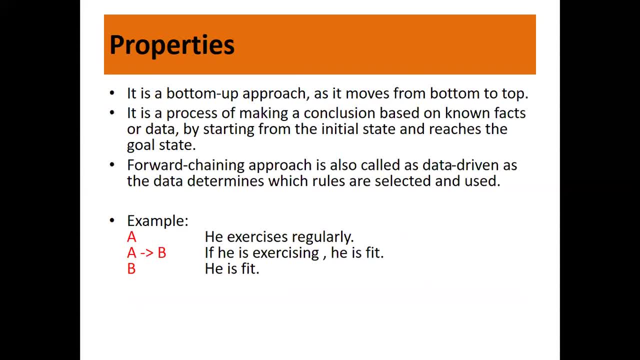 working memory. Now, what are the properties of forward chaining? It is a bottom-up approach as it moves from bottom to top. Why? Because from the bottom to top, it moves from bottom to top. forward chaining It is a bottom-up approach as it moves from bottom to top. Why? Because from the 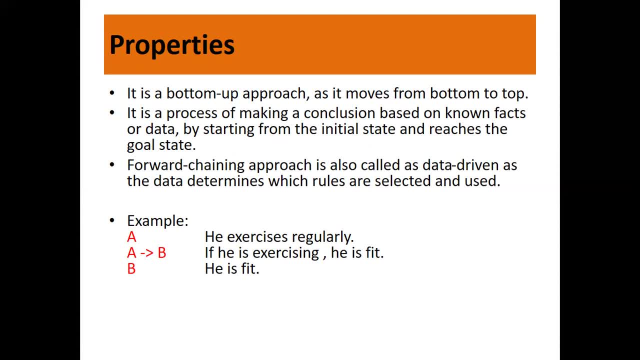 facts, we are reaching the goal. It is a process of making a conclusion based on known facts or data, by starting from an initial state and reaching the goal. state Forward chaining approach is also called as data-driven, as the data determines which rules are selected and used. So either data or 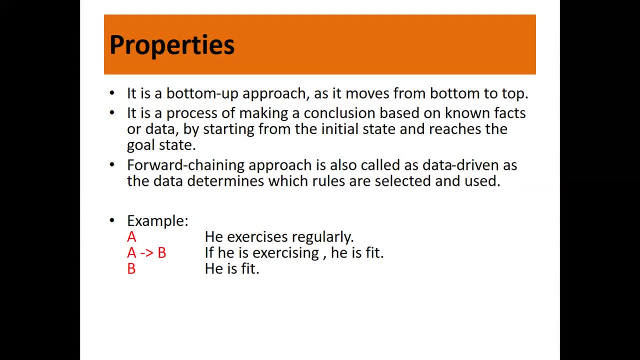 facts is given and you need to decide which rules you need to use for it. A simple example: if you can see what is the facts, we are reaching the goal. It is a process of making a conclusion based on known facts or data. So either data or facts is given and you need to decide which rules you need to use for it. A simple example: if you can see what is the facts, we are reaching the goal state and reaching the goal state, The fact given is that one 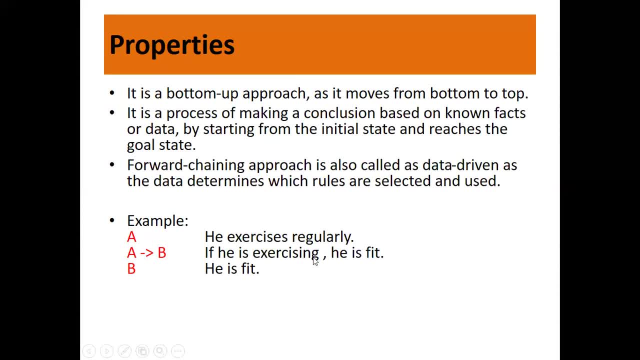 of the rules is exercises regularly, which means you need to exercise regularly as you need it. in the first order logic it is represented using A. Then the next rule. what is given is: if he is exercising, he is fit. If he is exercising that, A implies B. 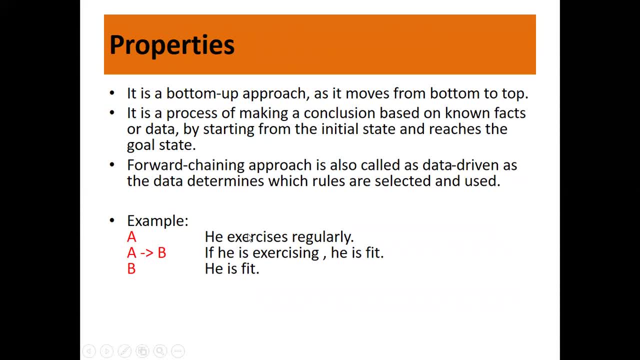 What is b? he is fit. These two things are given-. what is the new knowledge you could generate? The new knowledge generated is: he is fit, which can be added to the knowledge base. This is forward chaining. This is all for this lecture. See you in the next lecture. 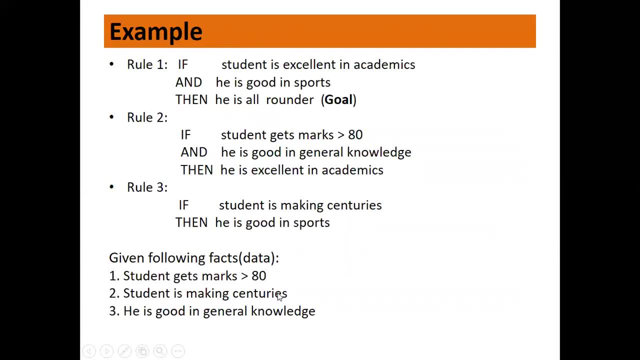 Right. We'll look at an example in detail, So the concept will be still more clear. Here I have the three rules given and the facts given. Right Now, using these three rules, I need to reach a goal. What the rule one says: if student is excellent in academics and he is good in sports, then he's all rounder. 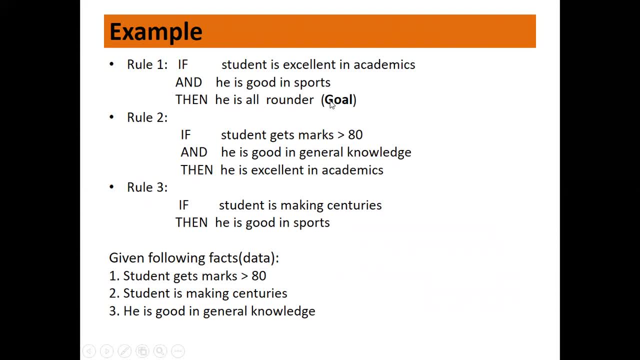 This is our goal. We need to prove that the student is all rounder Right. What the rule two says: the student gets mass greater than 80 and he is good in general knowledge, Then he's excellent in academics. This is the second rule. 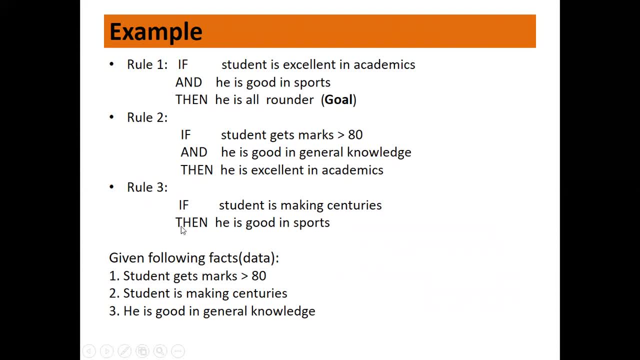 The third rule says: if student is making centuries, then he is good in sports. Now, using these rules from the knowledge base and given facts, what are the facts given? These are the three statements, or the facts or the data given is: student gets mass greater than 80.. 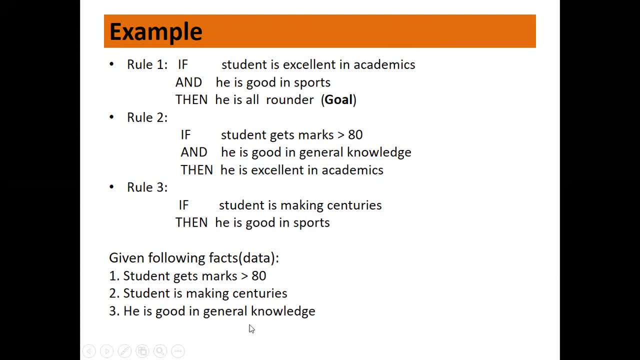 Student is making centuries. He is good in general knowledge. Now, given these facts, what should the goal? The goal should be: he is all rounder. So, using these facts, I should be able to infer that the student is all rounder. 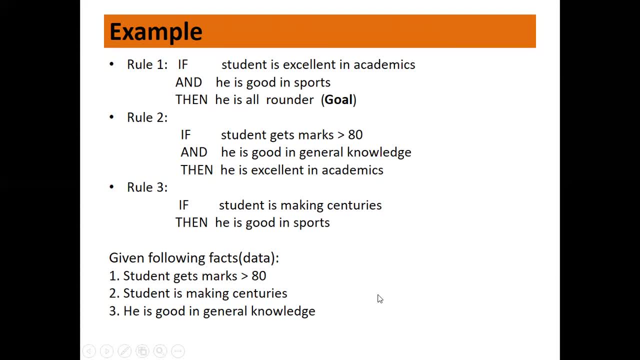 Fine, Let us see how we work with the forward chaining here Now, Here from these facts. what we'll be doing in case of forward chaining these facts will be checking whether they exist in the if condition right, Whether they are part of if condition. 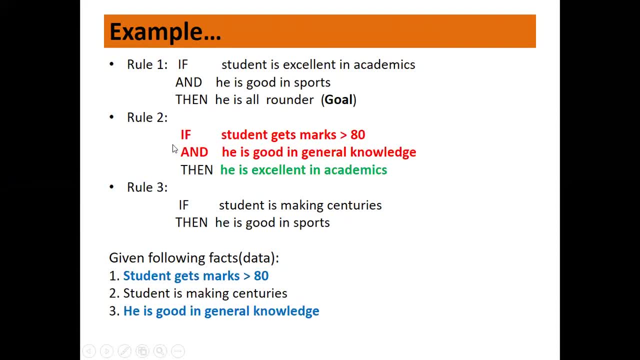 So let us go ahead Now. in rule two we already have these two facts in the if condition, If part of the rule, that is, student gets mass greater than 80.. So in the second rule we already have: student gets mass greater than 80.. 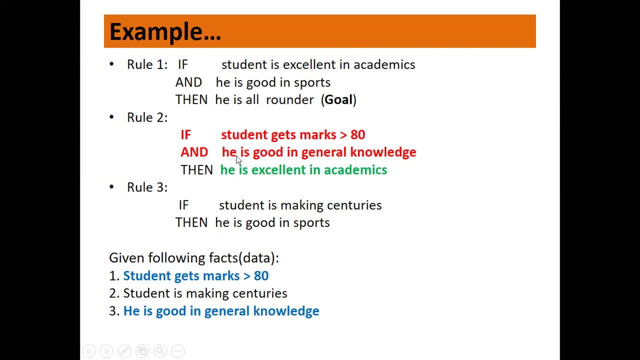 And the second fact that is good in general knowledge is also there in second rule two. He is good in general knowledge. So, given these two facts which are matching with our rule, what we get in the then part, he is excellent in academics. 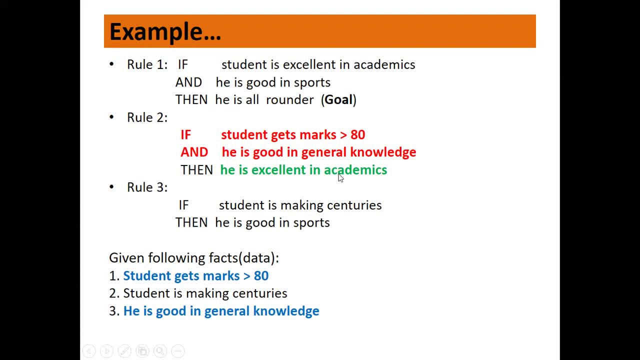 So this is subgoal. what we have got Subgoal is what He is excellent in: academics. So, using two facts, we could get a subgoal right Now. what is remaining Remaining is: student is making centuries. So we need to search whether we can get this fact in any of the, if part of the rules. 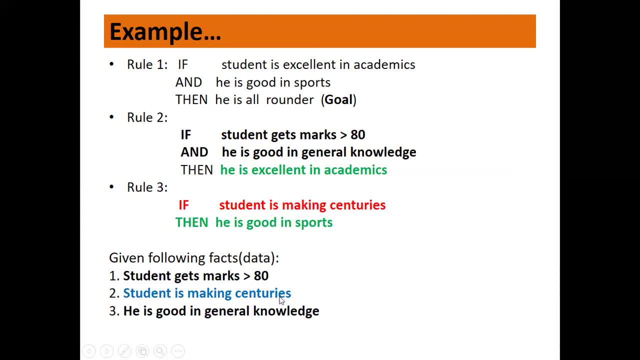 Now, if you look at rule three, student is making centuries. The given fact is part of the if condition here, right, And what is the subgoal here? Subgoal is: he is good in sports. Now we could get two subgoals. The first subgoal was: he is excellent in academics. 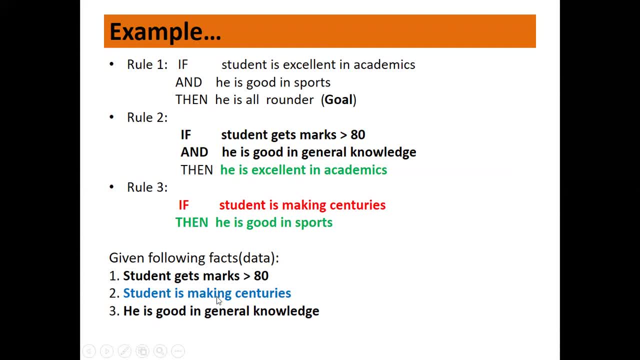 And the second subgoal is: he is good in sports. using these facts Now, using these subgoals, we'll try to get the goal Again, to get the goal, what we need. We need these subgoals to appear in the if part of the rules. 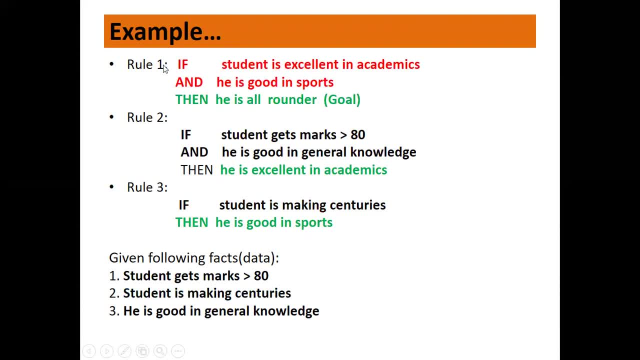 Now, he is excellent in academics. He is excellent in academics is already part of the rule one. You see, student is excellent in academics. He is good in sports is again part of the condition. He is good in sports. right? These two subgoals are appearing in the if part of the rule one. 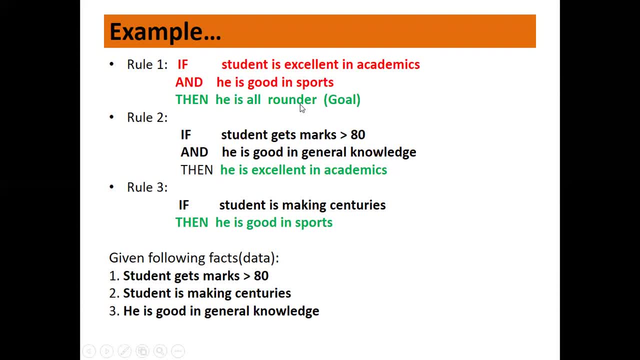 So we could achieve the final goal that he is all rounder. Is it fine If forward chaining using inference chain? I hope the concept is clear. What we did? We took these facts, We match these facts with the rules if part and then we got the then part as a subgoal and using these subgoals, 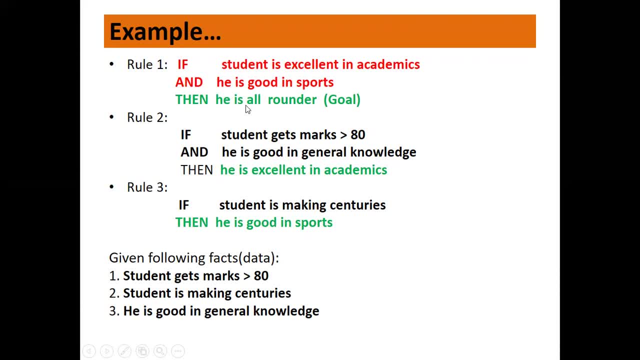 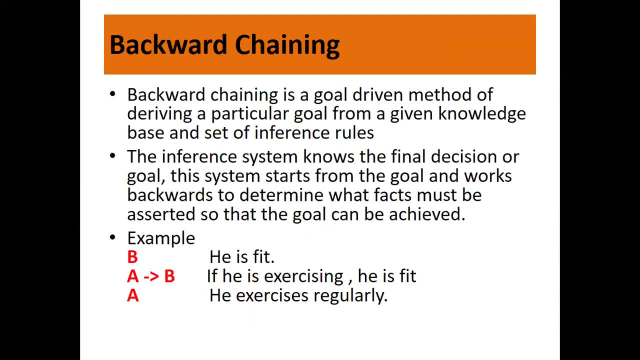 We saw these subgoals in the again in the part of the rules, and you could get the final goal. Fine, This is forward chaining. Now let us look at the backward chaining, which is exactly opposite of forward chaining. So in backward chaining is a goal driven method. 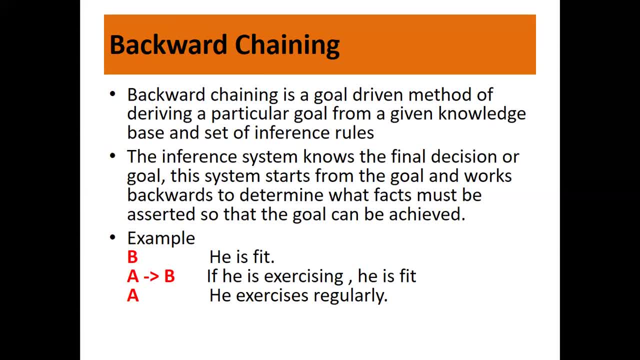 Whereas forward chaining was data driven method- Remember- backward chaining is goal driven method of deriving A particular goal from a given knowledge base and set of inference rules. The inference system knows the final decision or the goal. The system starts from the goal and works backwards to determine what facts must be asserted so that the goal can be achieved. 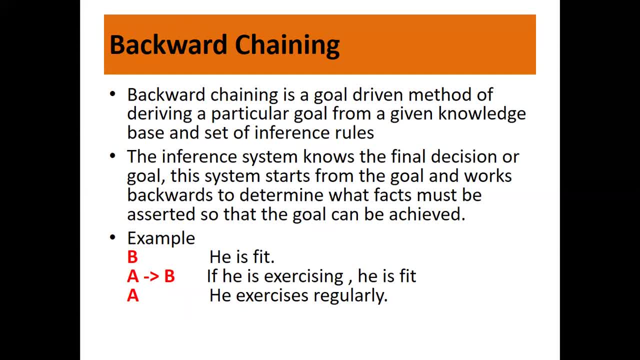 In case of forward chaining, what we did? we were given the facts and using those facts, we reach the goal. In backward chaining, you are given the goal, using the goal. You should go back to the fact using which you could achieve this. 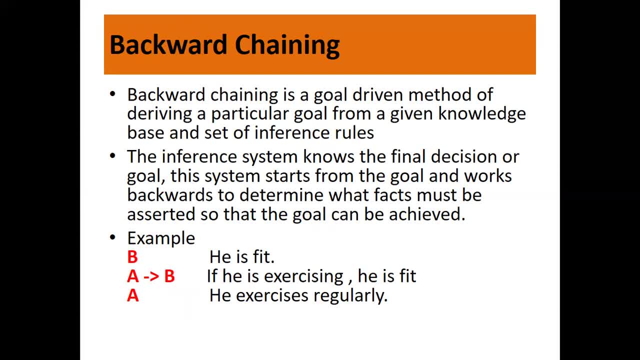 The simple example is the same as what we had in forward chaining. The goal is what he is fit. This is goal. So how do you reach what you need to find out? You need to find out if he's exercising his foot and he's exercising regularly. 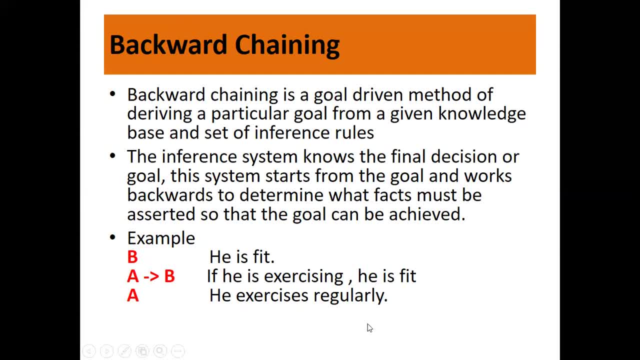 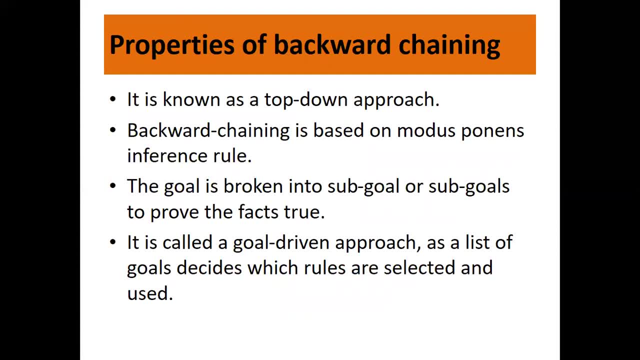 He exercises regularly. Is it fine? Now let us look at the properties of backward chaining. It is also known as top down. Why? Because we are starting from the goal and going Back to the initial state. Backward chaining is based on modus ponens inference rule. 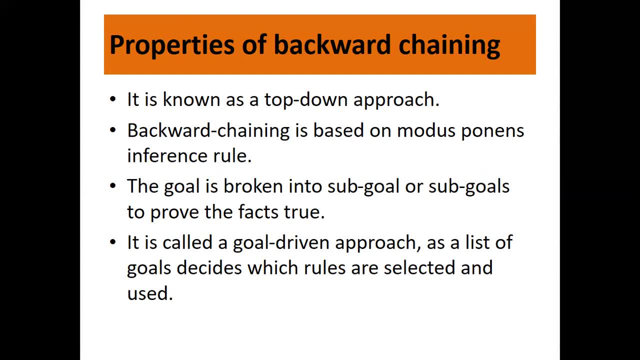 If you can recollect, forward chaining is also based on modus ponens inference rule. The goal is broken into sub goals or sub goals to prove the facts true, It is called a goal driven approach, as a list of goals decide which rules are selected and used in case of forward chaining. 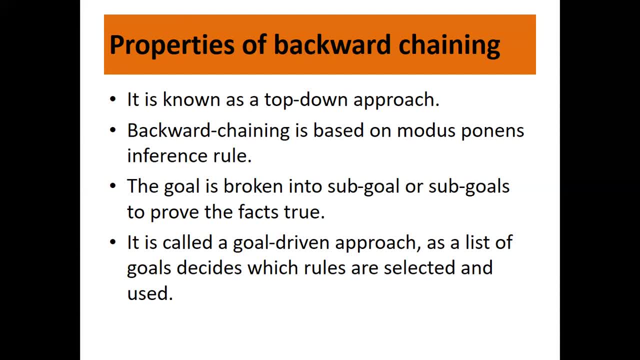 We had the data which is to decide which rules should be used, and here the goal will decide which rules should be. So in case of forward chaining, we used to match it with the if part. in case of backward chaining, we'll be matching the facts with the then part. 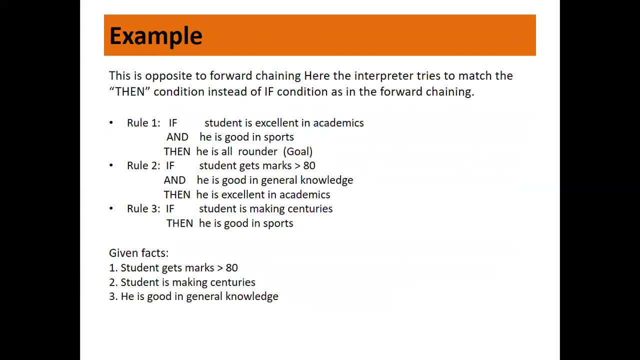 Right. So again the same example: what we had in forward chaining, but the approach is now backward chaining. So this is a positive forward chaining. here The interpreter tries to match the then condition instead of if condition as in the forward chaining. 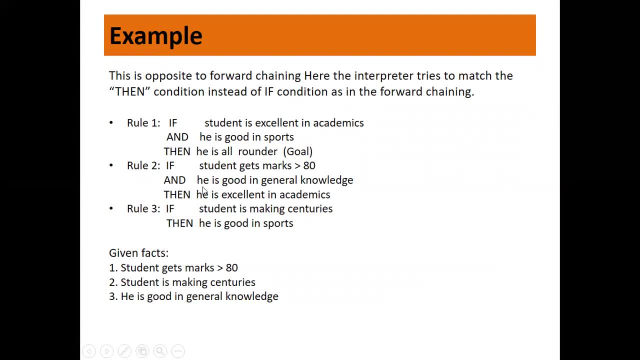 So again you have the students, the rules given And the facts given. now, what is the goal? goal is what he's all rounder using this. We need to prove these facts are true, right. So now, we are not starting from the facts. 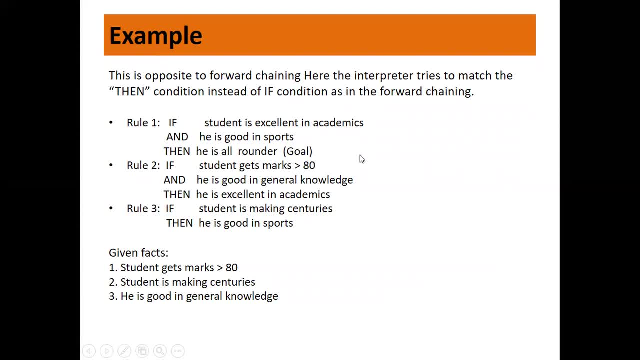 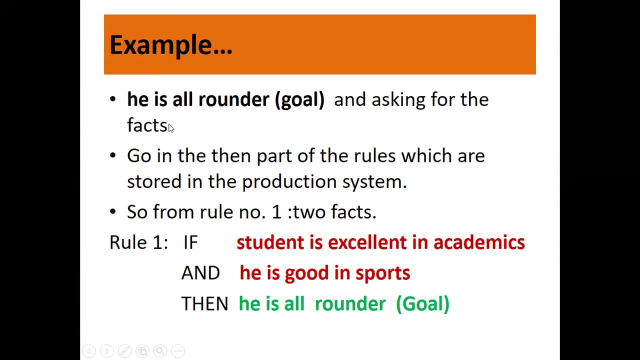 We are starting from the goal. So what is goal? He's all rounder right, So he's all around- is the goal And what we need to give them, we need to give the facts for this goal. So go in the then part of the rules which are stored in the production system. 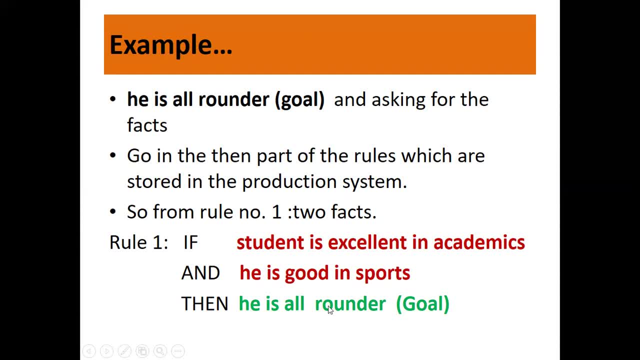 So let us look at the rule Number one. rule number one already has he He's all rounder, which is a goal, And what are the facts associated with it? It has two facts: Student is excellent in academics and student is good in sports, right? 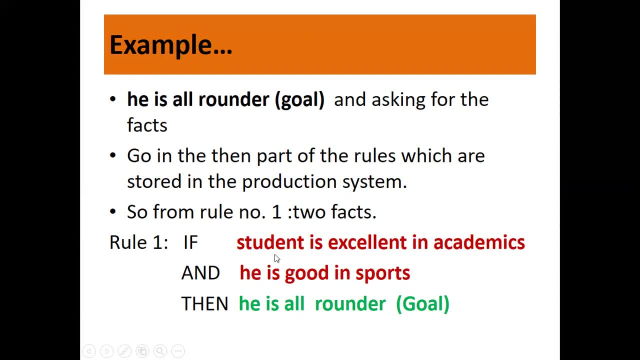 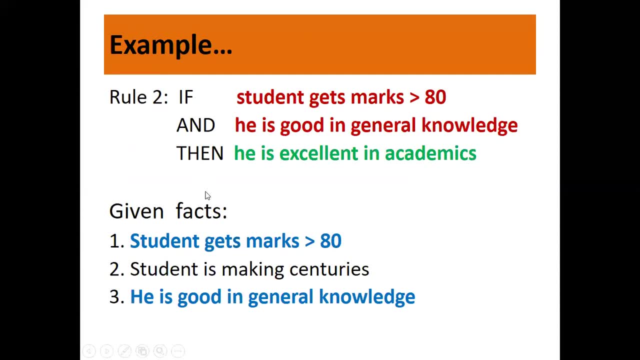 So from this goal, we could get two facts right Now. let us sell these two facts Now. these two facts, you can get it in rule number two. these two facts, we could get them in rule number two. right, What is rule? 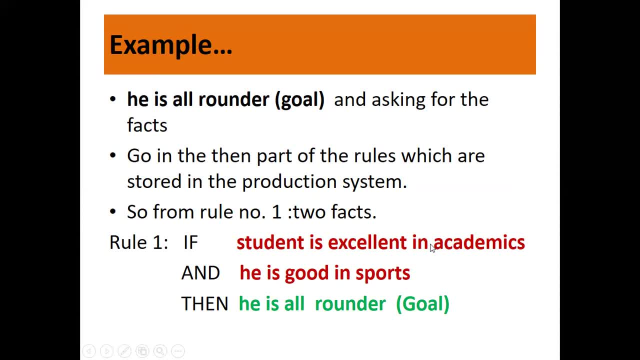 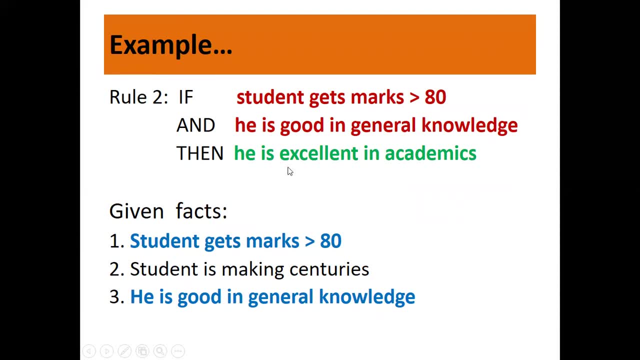 Number two, saying student is excellent in academics. This fact is now goal of the rule Number two: he is excellent in academics, So he's excellent in academics. You could read this goal Then. what are the facts? We support this goal. 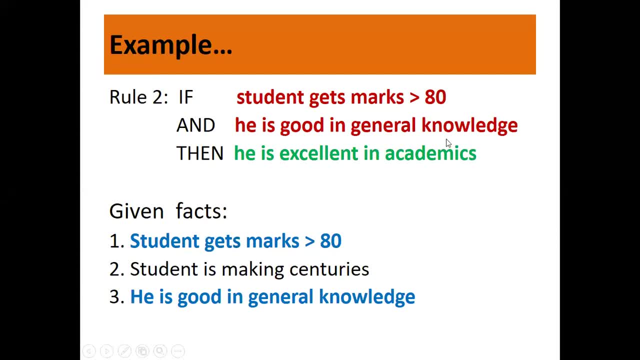 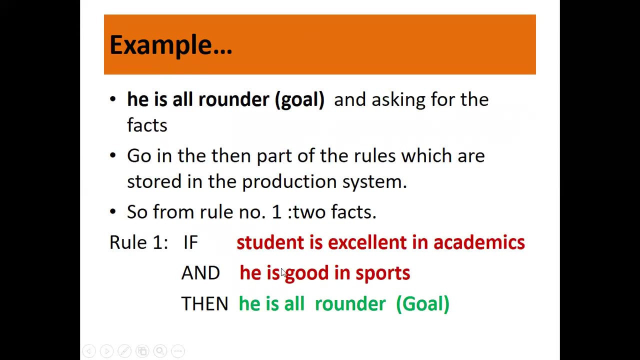 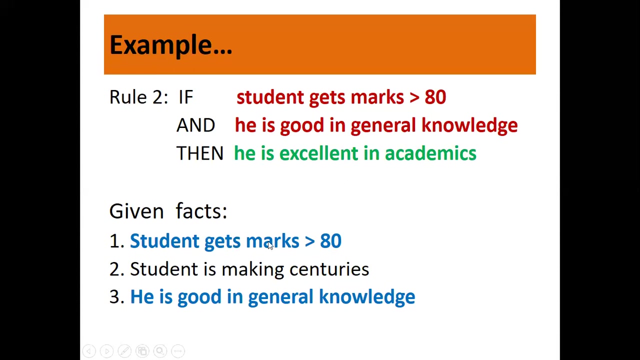 Student gets mass greater than 80 and student is good in general knowledge. right, So we could get now the facts: student gets mass greater than 80 and student is good in general knowledge. Is it fine What we did? we use? student is excellent in academics using this sub. if the part we could get two facts- student gets mass greater than 80 and student is good in general knowledge- using rule two. 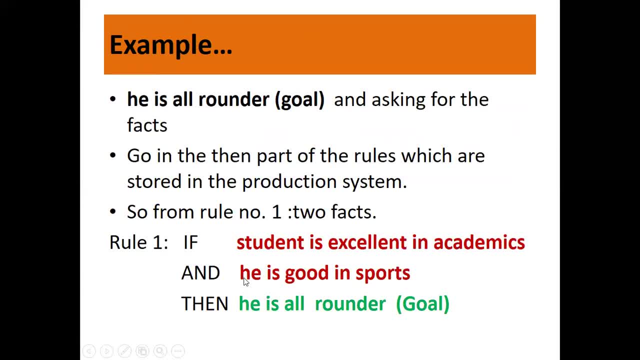 Now what we need to use- another- if part or the goal is sub goal- is: he is good in sports. Now let us search this: he is good in sport in the then part of the rules. Of course it is not in the First rule. 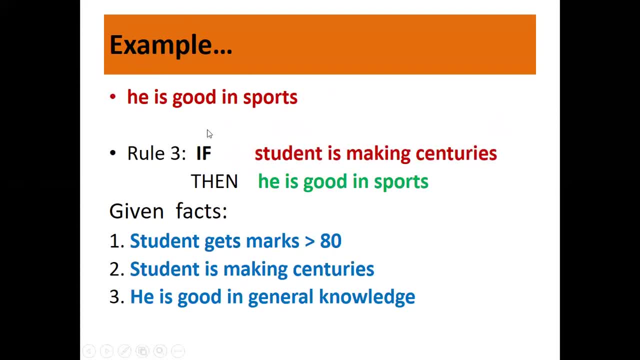 It is not in the second rule, So we move to the third rule is good in sports is in the goal. part of the rule three, That is: he's good in sports. So what fact we could get from here. The fact is: student is making centuries right. 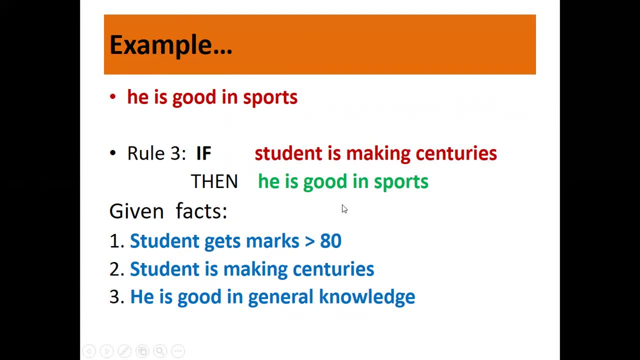 Student is making century, So starting from the student is all rounder. We could generate all the sub goals and reach the facts. We could prove the facts are a very simple example of backward chaining: right In Forward chaining we started from the facts and reach the goal in backward chaining.